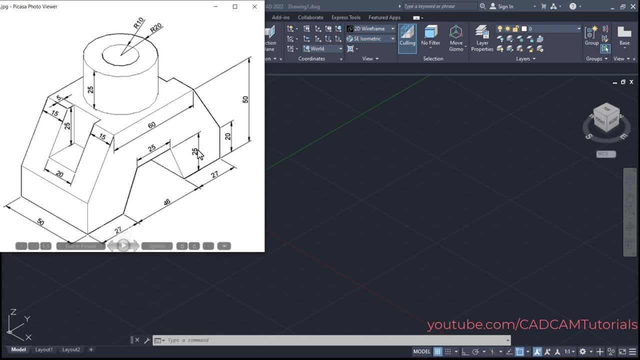 mirror it. So to create this base object, at first we will have to create this sketch. as this sketch is vertical, therefore, we will have to change UCS. right now, our XY axis is horizontal. we want it to be aligned with this face. so to work on. 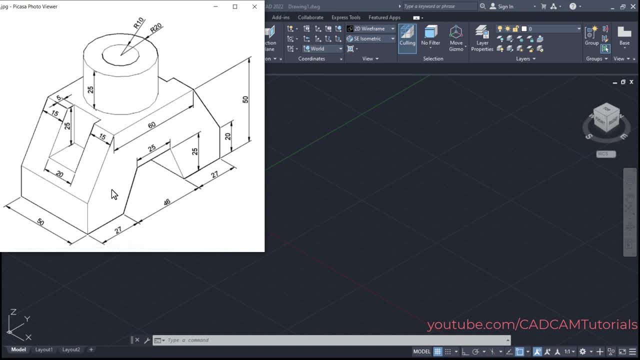 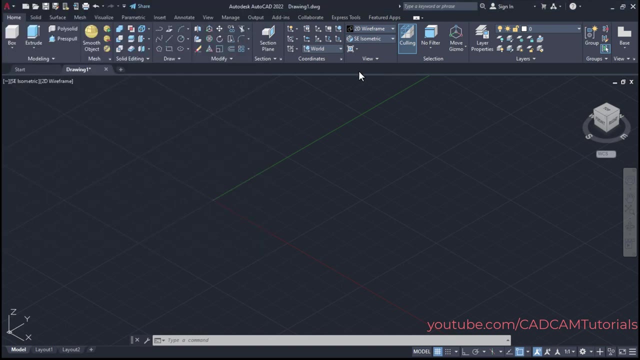 this face you will have to use the right UCS and if you want to work on this face you will have to use front UCS. and to work on this horizontal face you will have to use top UCS. so for this face we will use right UCS. so to change UCS. click here on world and click here. 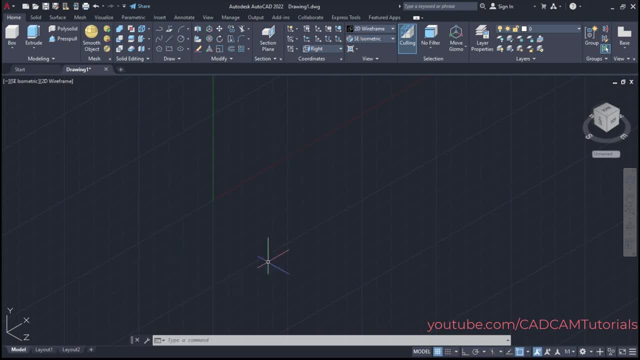 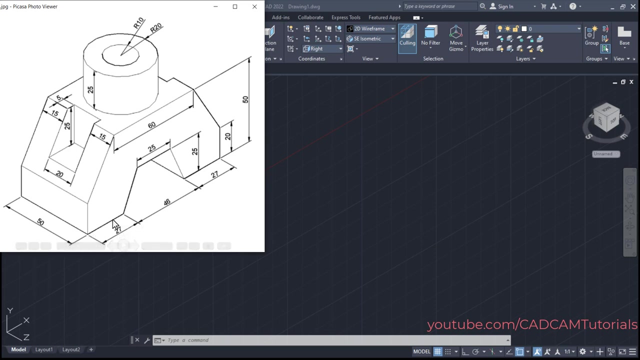 on right. so here you will see that plane has been changed and our XY axis is vertical and Z is horizontal. now we will start this sketch from this point. at first, we will create this line of my sketch for this point, and then, first, we will add theulital수. 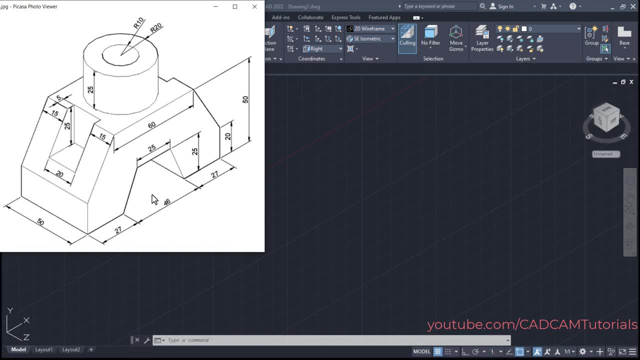 line of 27 size, then this line of half of this 46, that is 23. then vertical line of 25 and again this vertical line of 25, that is 50 minus this 25. that means this will be 25 and we will create this half line of 12.5, because we are going to create half portion. 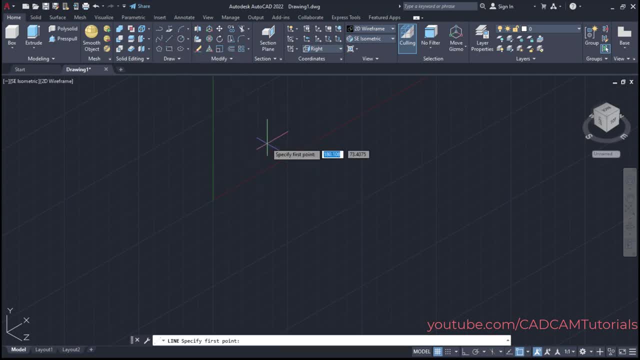 here on line, then you can start object from any point. Suppose I will start from 0,0, so type here 0,0, enter, then make children take your cursor on this side. specify length of 27, enter, Then zoom there again, take your cursor on this side. 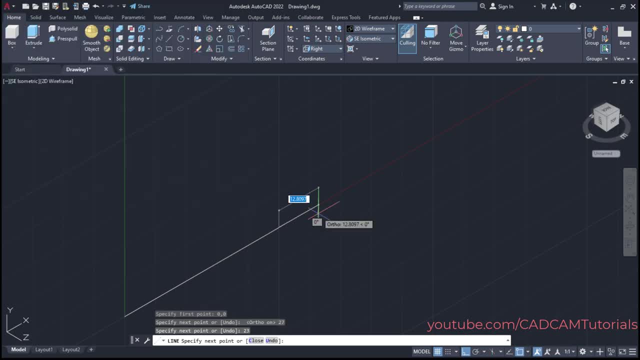 Then 23.. half of 46: enter, then take your cursor on this side. 25 enter, zoom minus. then take your cursor on this side. 12 and 5 enter, then click here on this end point. you can also make ortho mode off so that it will be visible perfectly. click here on this end point and press enter to stop line command. 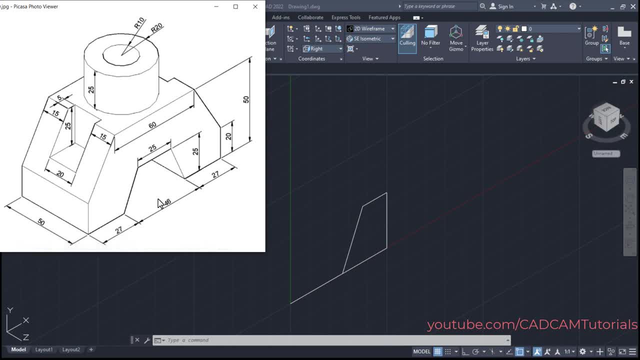 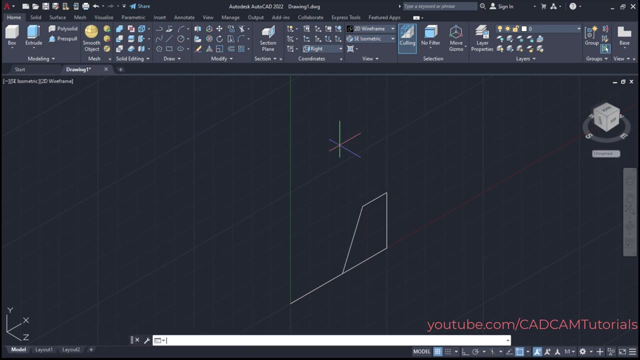 so here this shape is ready. then next is this line of 25 height, that is 50 minus this 25, and this line of 28. then we will create this line of 30 length, that is half of this 60. you can press enter to repeat last command. click here on this end point. 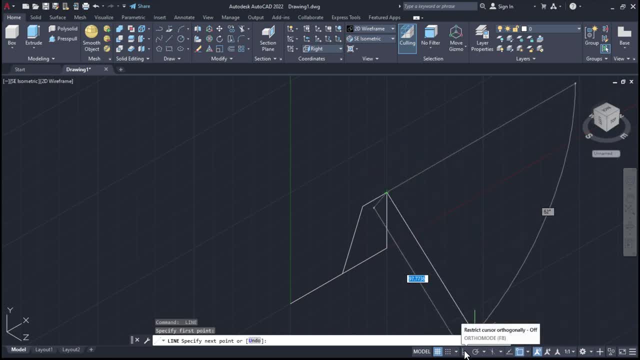 make ortho mode off. ortho on. take your cursor on this side. 25. enter. then take your cursor on this side 30 enter. enter again. enter to repeat line command. click here on this end point. take your cursor on this side. 20, enter and click here on this end point, press enter. so this sketch is perfectly ready. 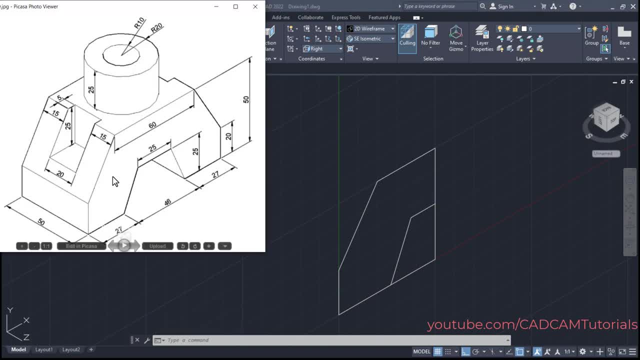 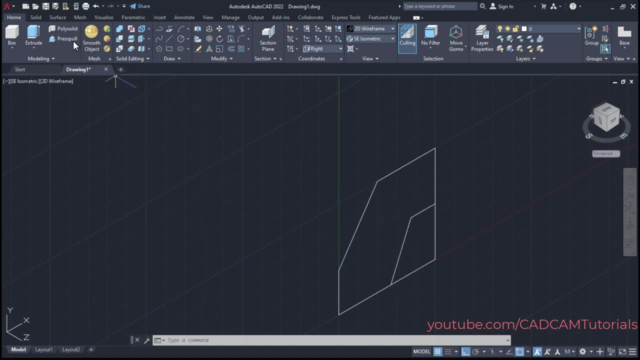 then next is to convert this shape into 3d. thickness of this part is 50.. to convert this object into 3d, click here on press pull. take your cursor inside this shape. once it becomes blue, click there. take your cursor on this side 50, enter and press escape to stop press pull command then to watch this object in 3d look. 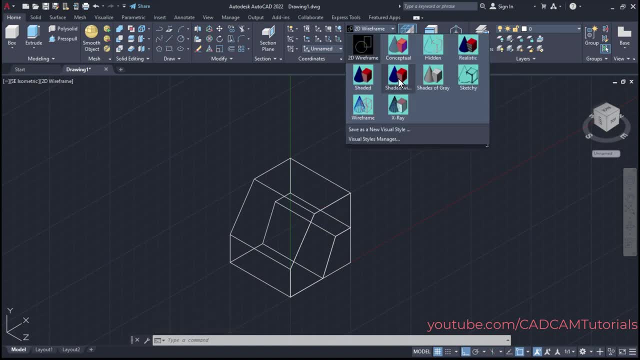 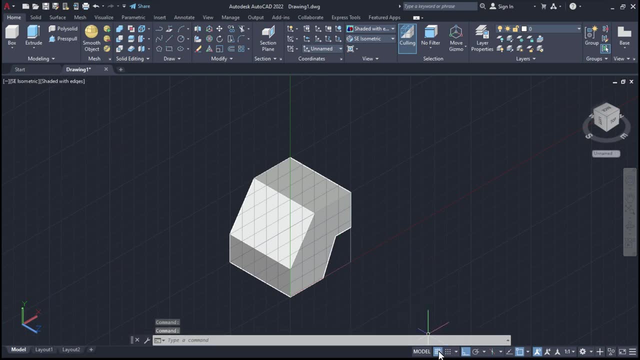 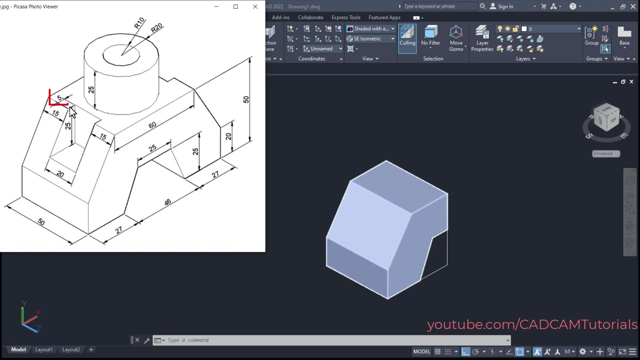 click here on 2d wireframe and click on shaded with edges, then i don't want to see these grid lines. click here on display drawing grid, so it will turn it off. so here this portion is perfectly ready. then next is to create this cut now. here this length is 5, then this length is 20 and 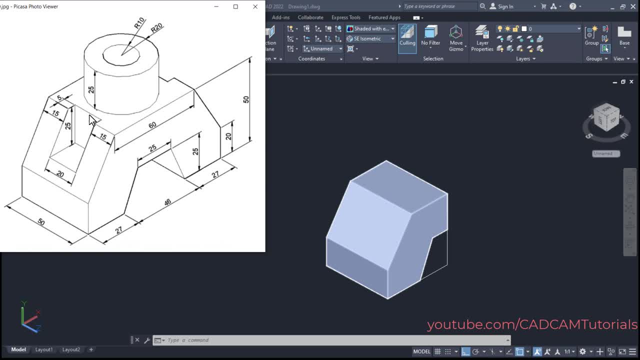 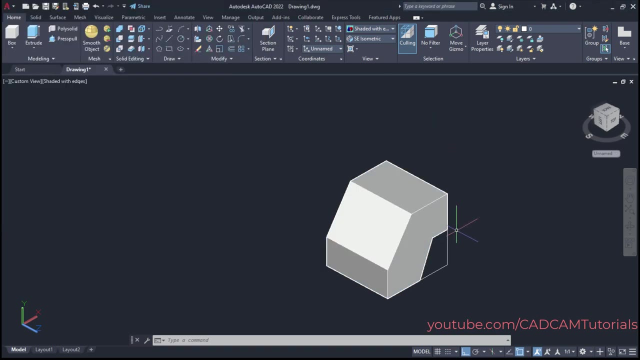 from either side it is 15. that means this object is at the center of this horizontal line. so in this, at first we will create this rectangle of 5 by 20 size, then we will press pull it by 25 depth. click here on rectangle, then click in empty space, take your cursor away. now, here we are on right place. 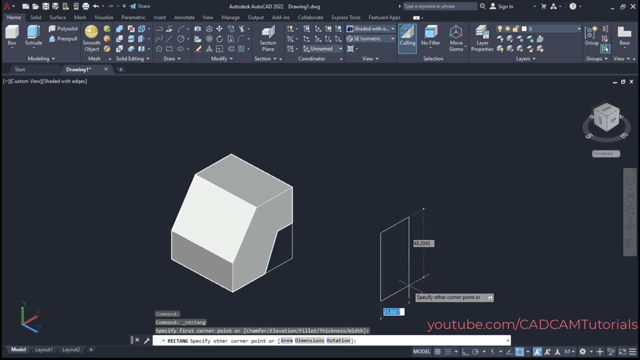 then click in empty space, take your cursor away. now here we are on right place. now here we are on right place. now here we are on right place. but now we have to work on top plane. so press escape and click here and click on top now here. 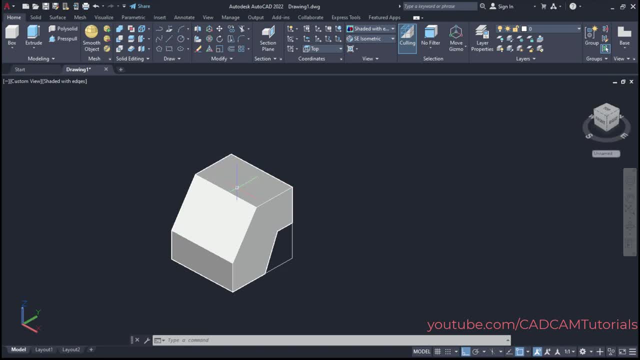 the XY axis are horizontal. that is parallel to this place. click here on rectangle. let me guess. click here on rectangle. click in empty space, take your cursor away, then specify year 20, press tab, then specify year 5, then press enter. then we will move this rectangle. 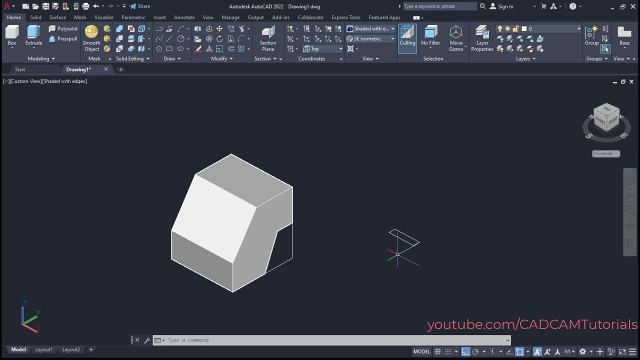 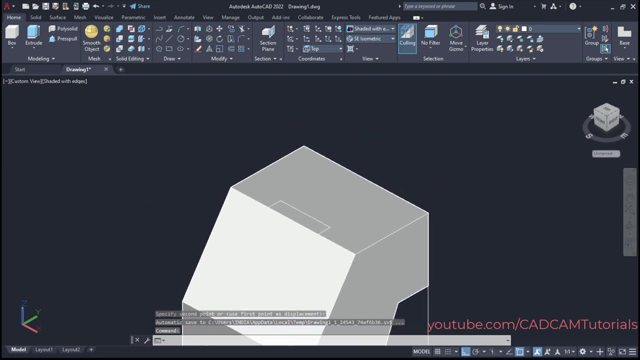 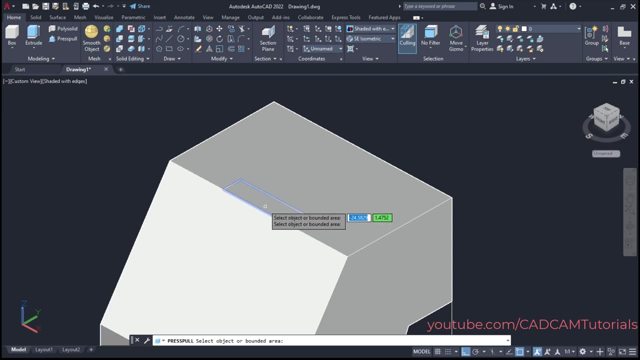 then specify year 5, then press enter, then we will move this rectangle and place it here. for that, click here on move. select this object, press enter, then base point will be this midpoint: click on it and click on this midpoint. so here it has been placed perfectly. then to cut it again, click on press pull. click inside this shape. take your cursor. 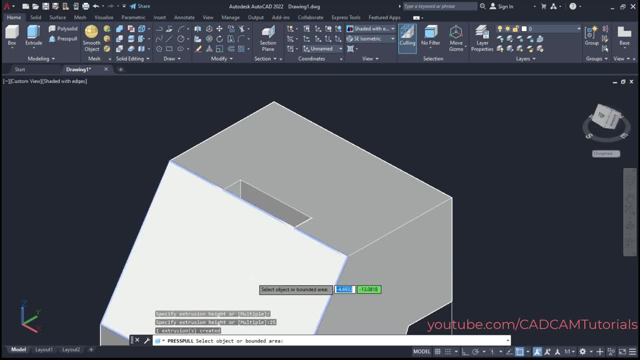 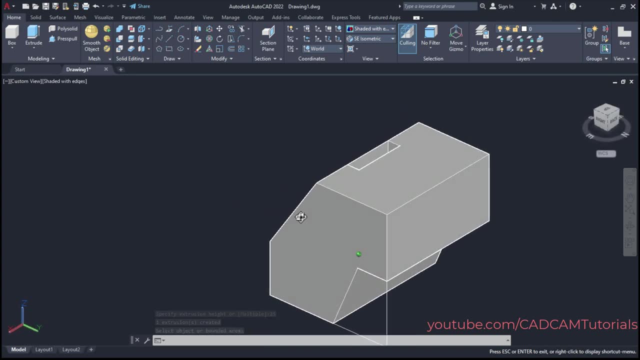 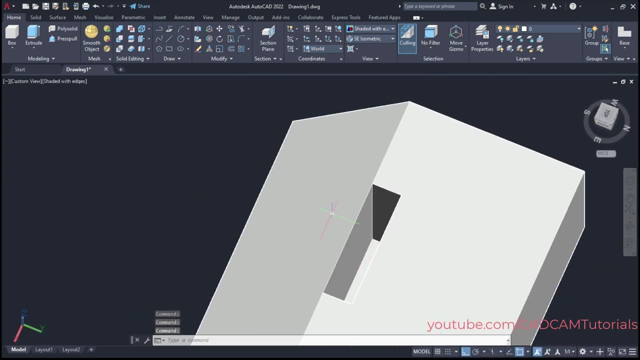 below. specify depth of 25. enter press escape, then orbit it, press shift, press middle mouse button and drag the mouse. so here this cut has been created perfectly. then we will have to cut this complete portion. for that, click here on press pull, then take your cursor to. 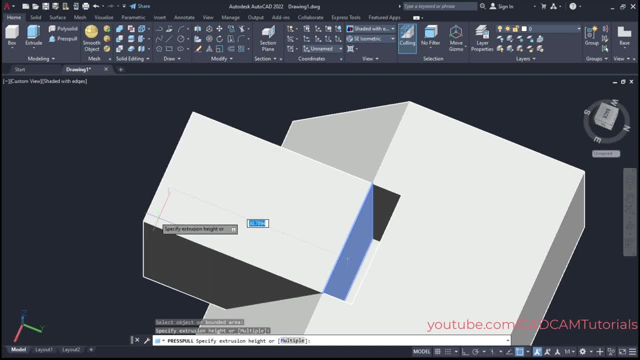 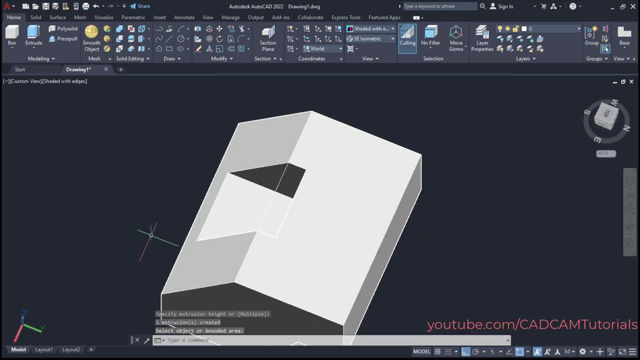 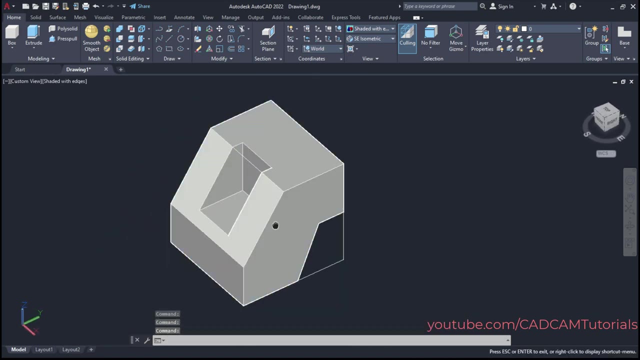 this vertical rectangle. click there, take it outside, ensure that you are coming out of this object. click, press, escape, then orbit it. so here this cut has been created perfectly. then remove these unwanted lines for that type E: enter and select these lines. enter. then we want same shape on the opposite side. so for that, 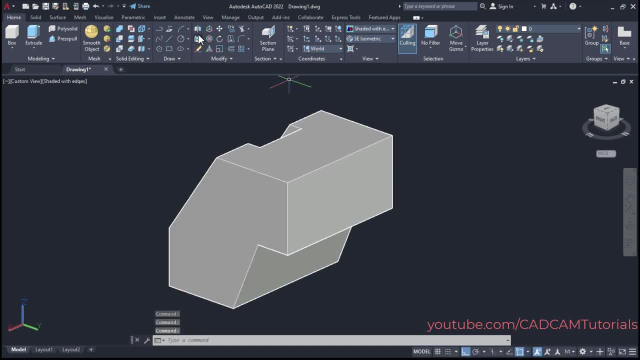 we will mirror it. click here on 3D mirror. select this object, enter. then we will have to specify three points of the plane around which we want to mirror. so we will have to mirror around this plane. so select three points of this plane. I will select this end point as a first point. this. 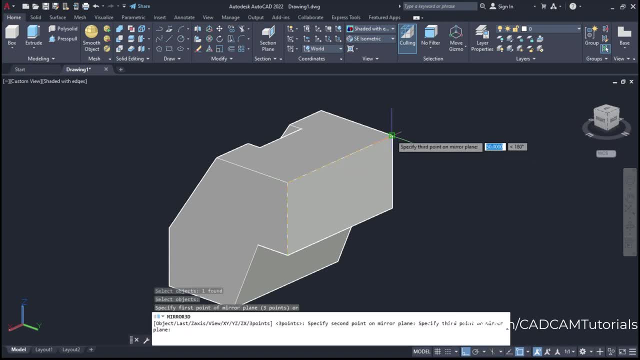 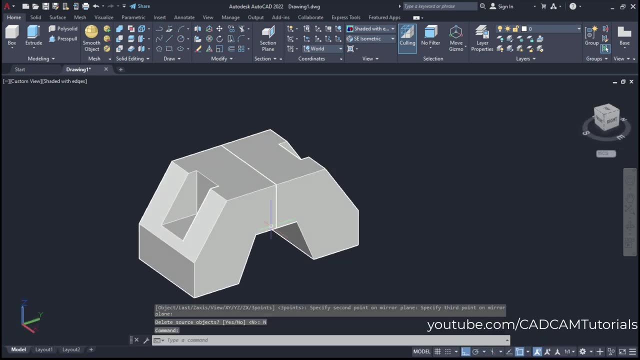 end point as a second point and this end point as a third point, then select this end point. so here this mirror is created. now these two objects are separate. we want them to be connected. for that, click here on solid union, then select this object and this object and press Enter. okay, it was not selected perfectly. again, I will. 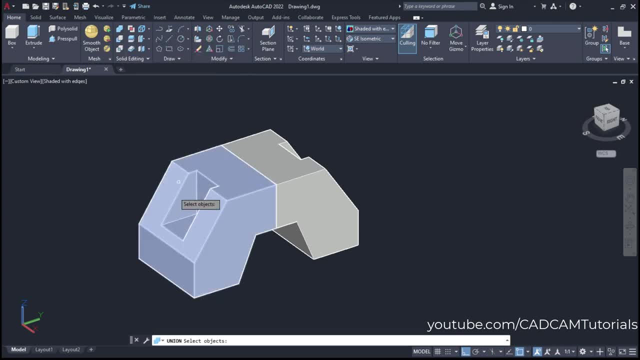 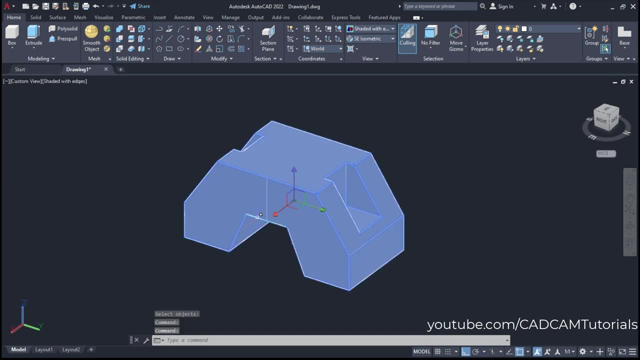 select here on solid union. once it becomes blue, click on it and this one, press Enter. so here this object has been connected perfectly and I don't want this line here. I am not able to select this line. so what I will do for easy selection: click here and select this 2d wireframe in 2d wireframe. it is very. 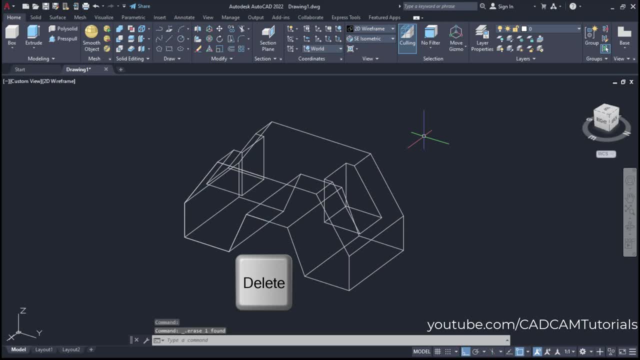 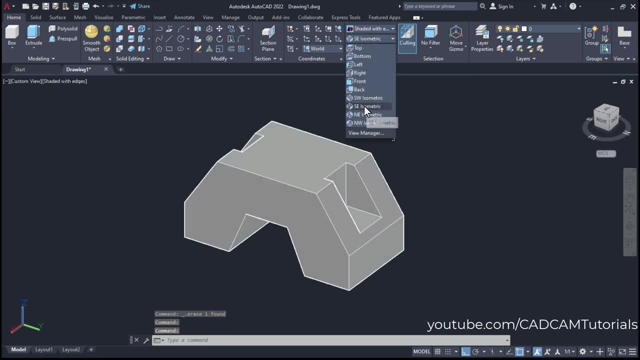 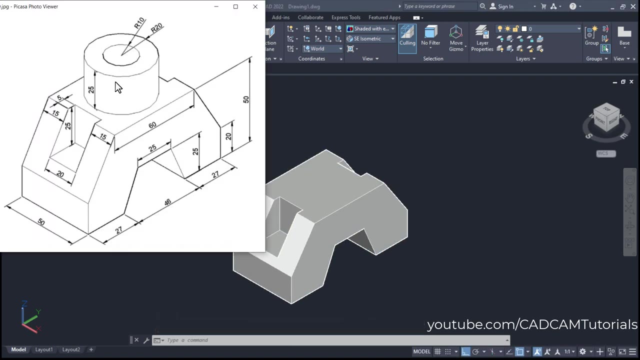 easy to select unwanted objects, then press delete again, click here, click on shaded with edges and click here on SE isometric. so here this object is perfectly ready. then next is to create this cylinder of 10 and 20 radius and 25 height, and this internal cylinder is actually a through hole. 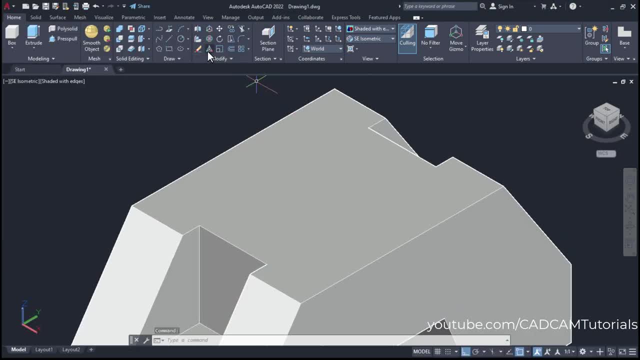 so zoom there, click here on circle center radius, then take your cursor to this midpoint, then this midpoint. now, because of dynamic UCS- actually we are not able to select it perfectly- so what we will do? we will turn off that dynamic UCS. but here dynamic UCS is not visible. to make it visible, click here on these three lines. 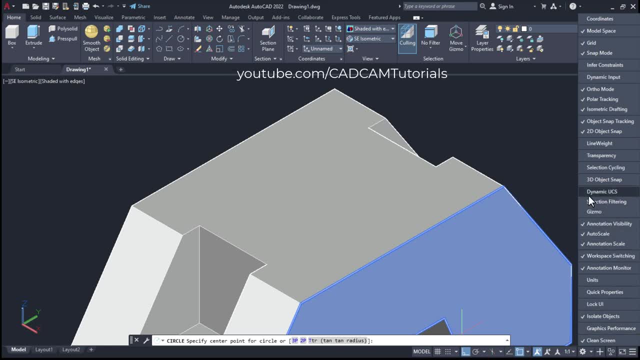 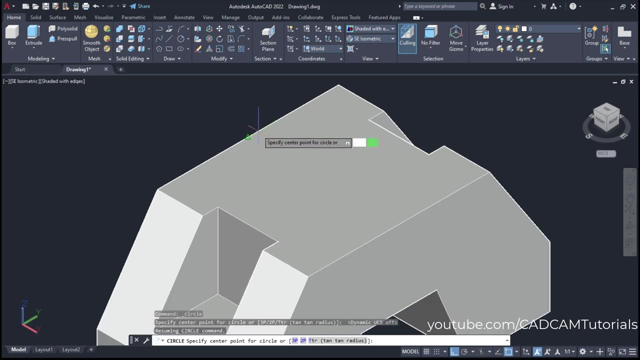 customization. and here is dynamic UCS. click on it, click outside. so here dynamic UCS is show, just click on it so it will get turn off as it is turn off, so it will not select that plane automatically and it will be easy to work. then take your cursor to this midpoint and one more.